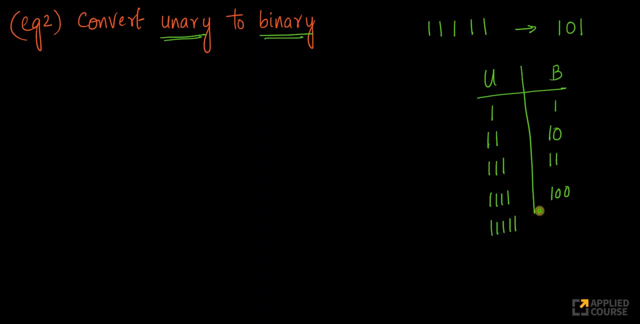 3 is this, This is 4.. If you have 5 1s, it should become 1: 0.. So this is basically base 2.. This is base 2 and this is base 1.. Now, how do we do this? 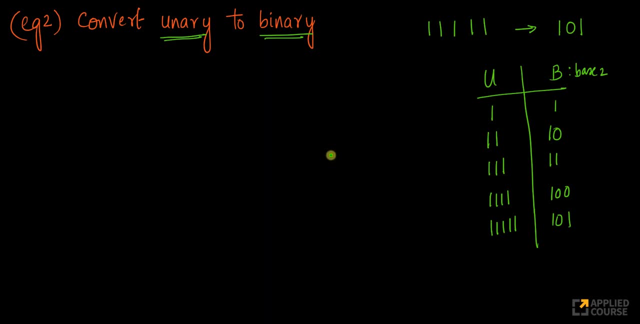 Okay, let us try to construct a Turing machine for this problem. So now, in my binary, instead of using symbols 0 and 1, look at this: For my unary- I will use the symbol 1.. To avoid any, 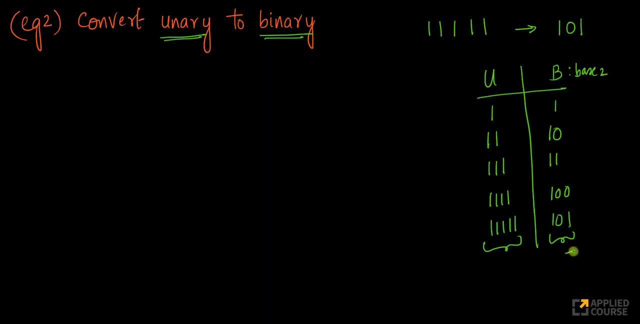 confusion. instead of using 1 and 0 here, I will use z to represent 1.. I will use y to represent 0 here. okay, Just for simplicity, To avoid the confusion between my unary alphabet and my binary alphabet, right? So this will. 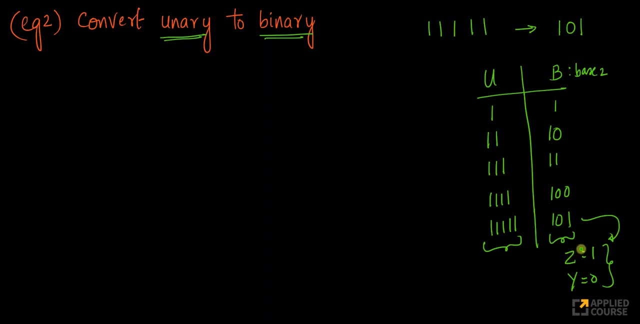 be in 1s, but the output will be in zs and ys, but z equals to 1 and y equals to 0. And how would my input look like? My input will look like this, right, So I have a blank. 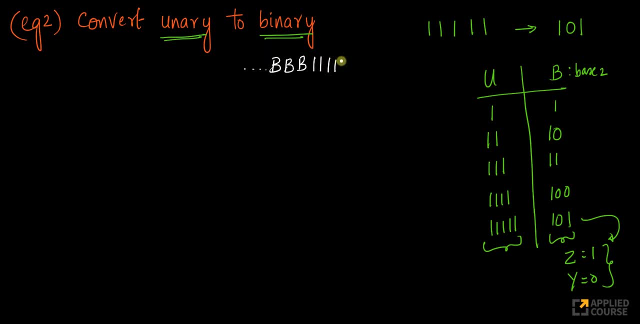 I have blank spaces. Let us assume my input consists of 5: 1s- right Again. then everything will be blanks, right. So this is my input string. Now let us start constructing the whole Turing machine for this step. 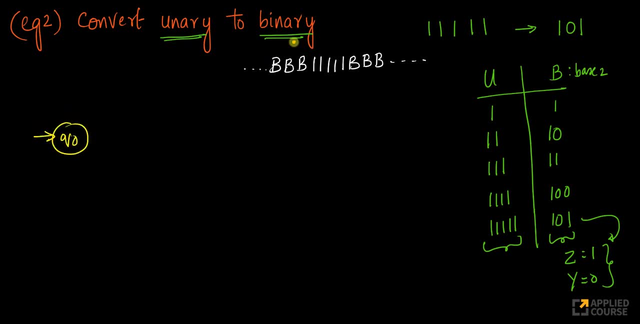 Step-by-step. So I start in state q0.. So my point, my read-write head, is here. I will start reading it now, okay, So what I will try to do. again, the logic here is okay. 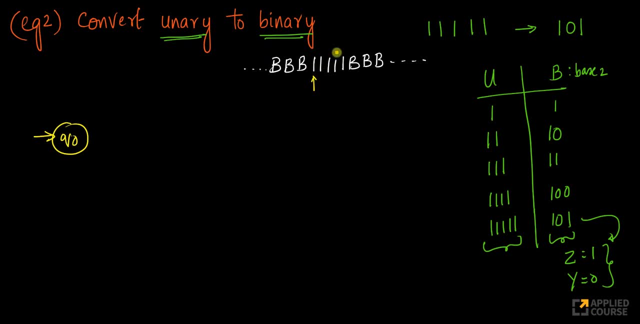 so the very important logic here is as follows: right, So while I am reading my input here, where would I write my output? This is where I am reading my input from. Where should we write our output? We can either write our output in this space or in this space, So 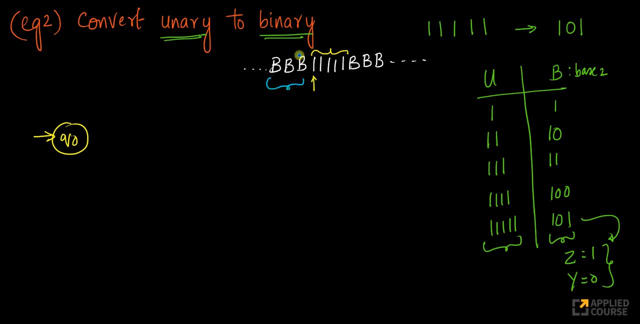 we will design a Turing machine which writes outputs on the left-hand side of the inputs. This whole thing is my input. My read-write header is always on the leftmost symbol of the input and I will try to write my output here, right? So let us go step-by-step. So how will I design this? 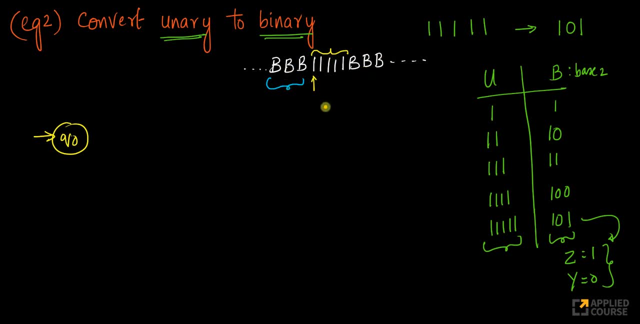 Again, there are multiple Turing machines you can design. What I am designing here is just one of the many Turing machines you can design that converts unary to binary. So this is my input and I want my output to be here. You can design a Turing machine. 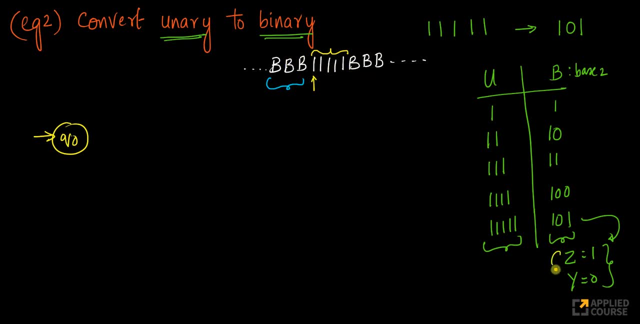 where the output is on the right side, right Here, to simplify the problem, I am using Z to represent 1,, Y to represent 0.. You could also create a Turing machine whose output is also in 1s and 0s instead of Zs and Ys. There are many ways you can construct it. I am trying to pick. 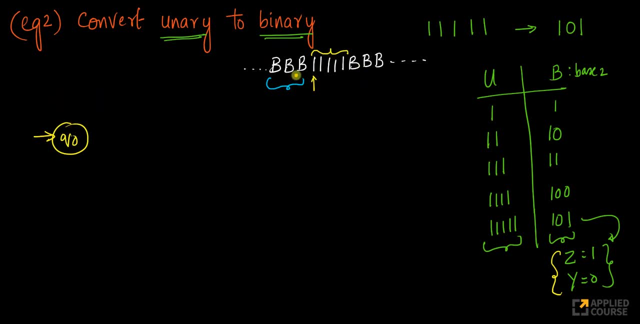 the simplest possible way. Okay, So let us go here. So I start here. Look at this. I start here Now if I encounter…. So the way I will think about it is this: okay, So the moment I 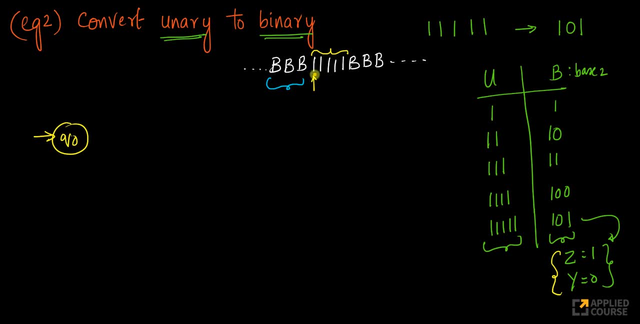 encounter a 1 here. see, I am reading this right. So what is the equivalent of unary 1?? Unary 1 equals to binary 1.. What is binary 1?? When I am using Z and Y here, this should be equal to Z. 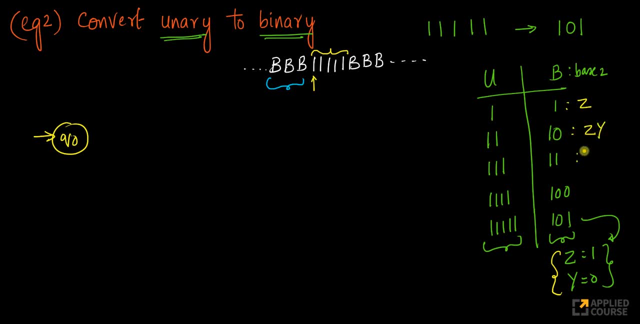 What will this be equal to? This will be equal to ZY. This will be equal to ZZ. This will be equal to ZYY. This will be equal to ZYZ, right, So on and so forth, Because I am using Z for 1. 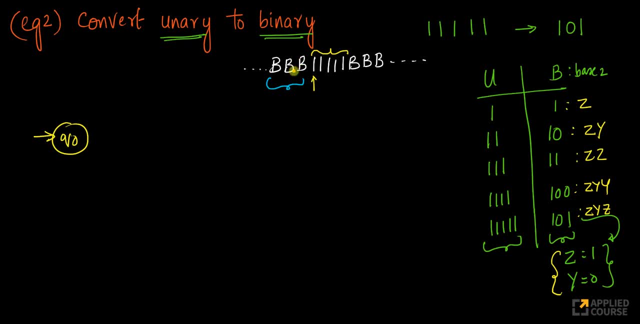 and Y for 0.. The moment I write, I read 1,. I want to write the output here, right? So let us go this way. So, for example, imagine if I am reading a 1, right, I read a 1 here. The moment I read a. 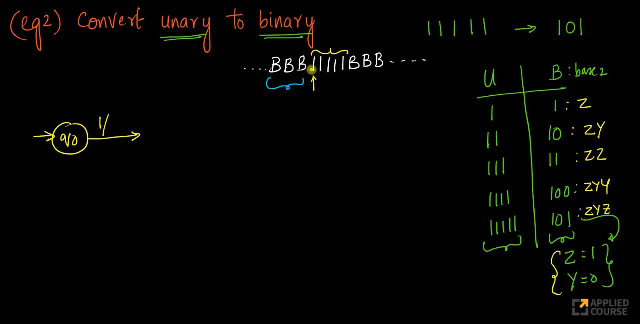 1,. what do I want to do? right, Because I have already read 1,. I want to convert this blank space into Z, which is nothing, but which is the corresponding base 2 value or binary value corresponding to whatever I have already read, right? So what I will do here is I will start. 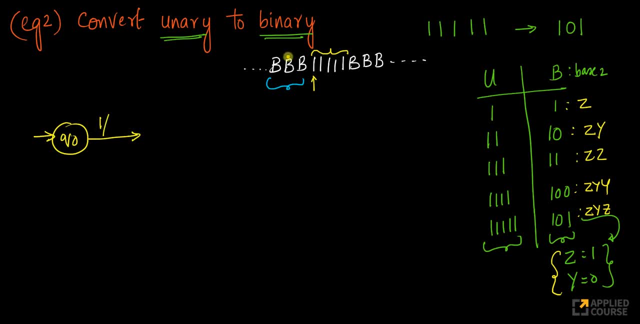 saying: if I have 1 here, if I have 1 here, I will replace this 1 with X, Because I I want to mark that I have already read this right. I want to mark the fact that I have already. 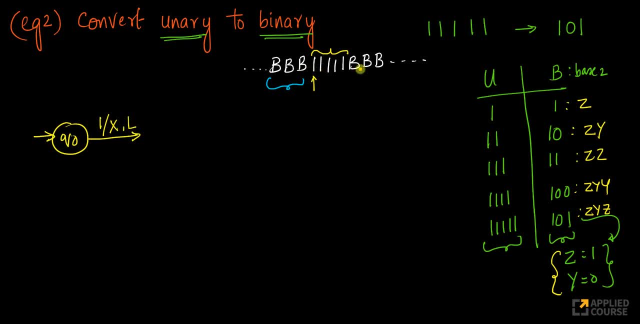 read this right And I want to move left. So now what happens here? This 1,, which I have already read, will become X. So let me change this to X, right, And I will move left, right. So what will? 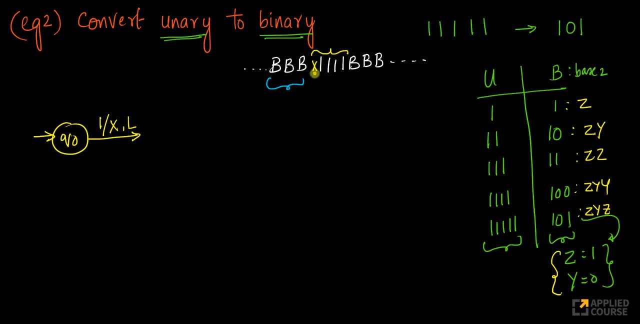 happen here is this, So this will become X. I want to mark the fact that I have already read this 1, right, So I move here now. right, Look at this. I want to mark the fact that this 1 has: 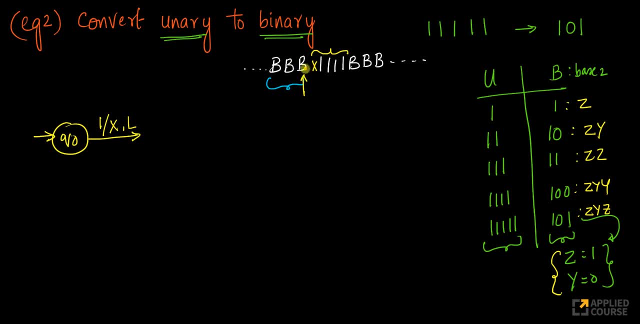 value. I want to place it here in in place of this B right. Very, very simple here. So now I have, I have reached my state Q1.. Now, what should I do? I should now. now, if I encounter a B here. 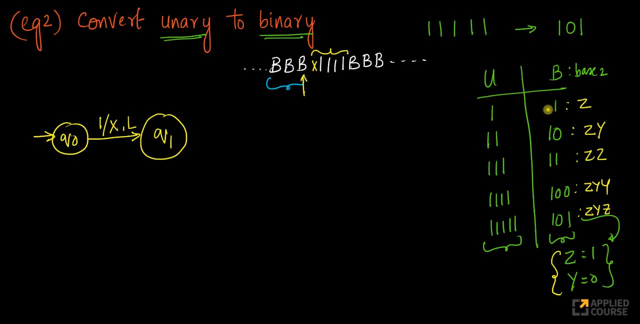 what should I do? I should replace this B, because I encountered a 1 here. I should replace this B with a Z. So let us write that logic here. right, If I encounter a B, I will replace that with Z. 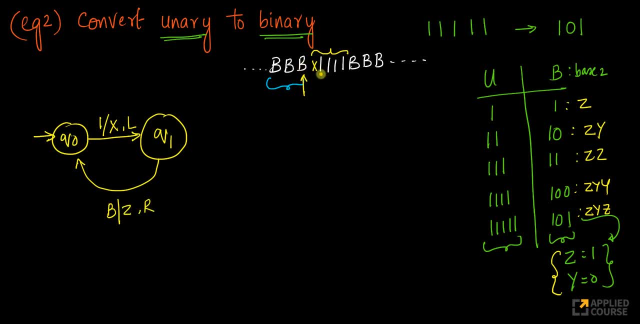 right, And I will move right now. I will move right, okay, Simple. So I replaced this B with Z. Okay, look at this. I, I am replacing this B with a Z. So what happened here? I have read the single 1.. I have also written its corresponding base 2 or binary value here. 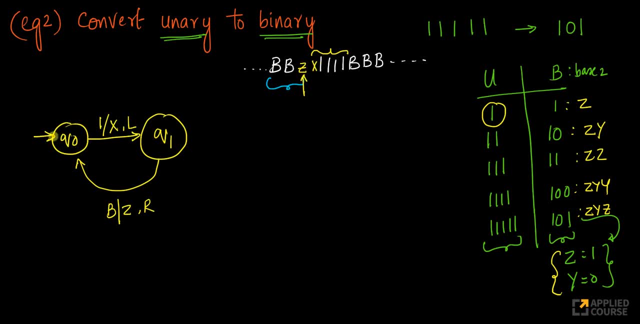 Cool. Till now, everything is working well. Now, now. now, what happens here? Look at this. Now, when I move right here, what happens? Look at this. It says move right because I have already written this value, So I move right, which means I am here. Now, when I encounter X, what should I? 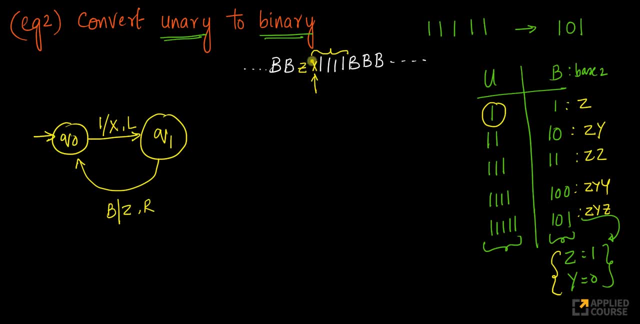 do? I should just ignore it, because that 1, has already been processed. The 1 that was initially here, that has already been processed and its corresponding binary value has already been written here. So I will just ignore this X here. right? I will simply ignore this X. So I will continue to stay in the same state. I will. 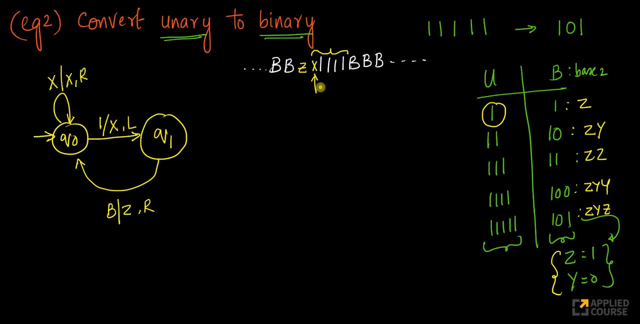 replace X with X and I will move to the right. right, Everything is looking good enough. Okay, let us continue. So again, we can easily construct Turing machines with examples. Again, what am I doing here? I am just taking some examples and I am trying to construct Turing. 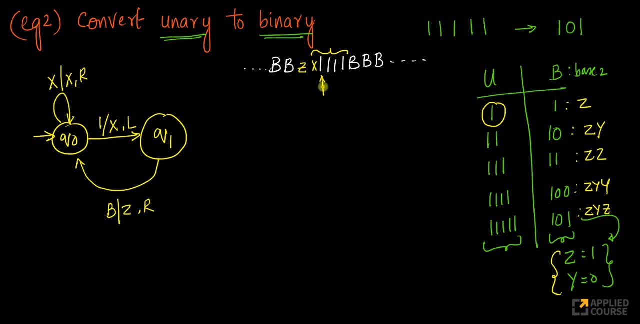 machine. Right, I am trying to go through each example and I am trying to do this. That is all I am trying to do. Now. imagine if I have this 1.. Now what happens on 1? I replace this 1 with X. Look at. 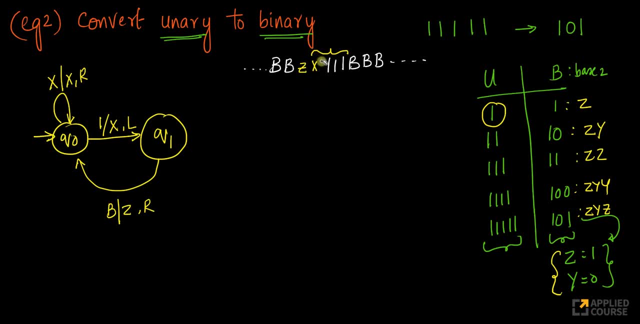 this And I move left. So what will happen here? This will be replaced. This 1 will be replaced with X. This 1 will be replaced with X, and I move left- Right When I move left. now look at this. 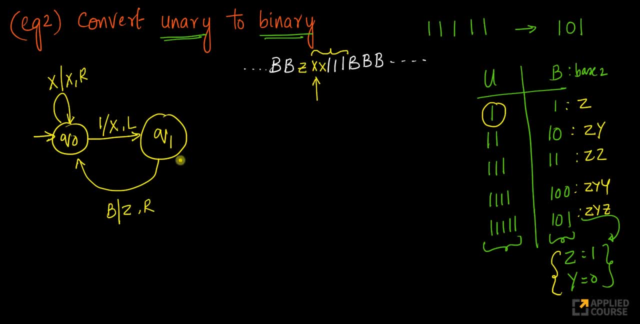 I have an X here, So this X has already been processed. So I am in this state right now. Now, if I encounter X, what should I do? Just ignore this X And keep moving left, Right Again? some people write these transitions, So I am writing this: 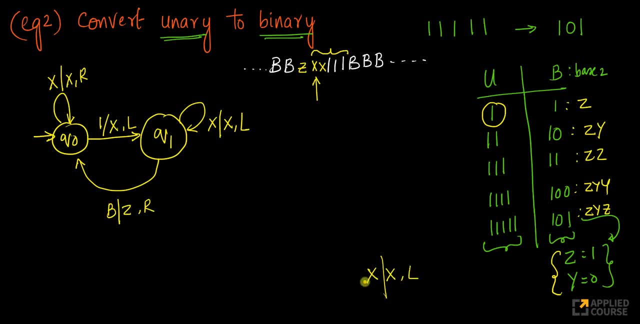 transition as follows: Replace this X with X and move left. This is how I am writing it, Because this is easier to read. Replacing this with this and moving left. Some people also write this as XXL, This triplet. They also write it like this, So there are multiple, depending on. 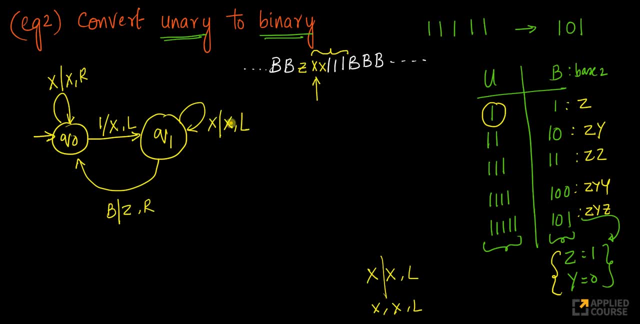 which book or which articles you are following, this representation might change. Some people also have seen write this as X comma, X by L, So there are multiple ways of writing this. So if you are reading a textbook where this notation or this notation for each of these transitions, 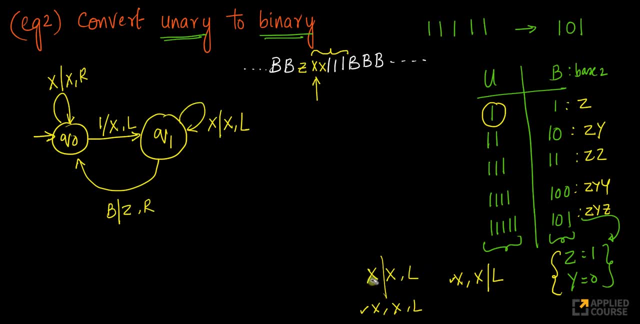 is mentioned. please do not worry about it, The concept is the same. The concept does not change Right, It is just a notational convenience. I prefer this notation because I can read this as X being replaced by X and moving left. I prefer this notation, Right. So now what happened here? 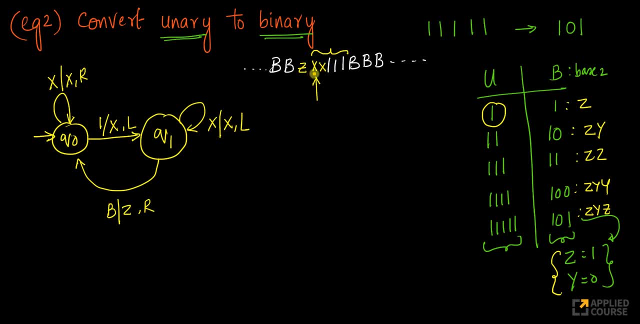 Look at this: X with X and I am moving left, Right. So where was I? So I replaced this X. I am in this state, So this should move left now. Look at this. This will move left now. So I am at Z Right. 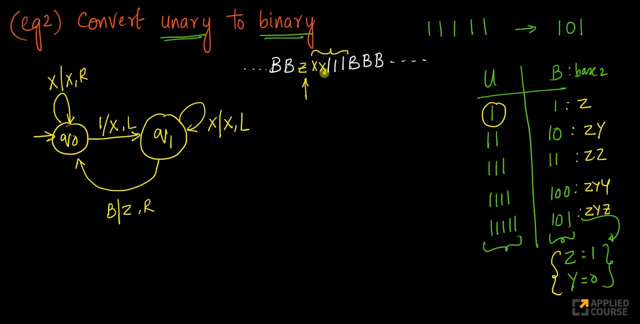 I am at Z now. Right Now, if I get a Z, what should I do? Look at this: Now I have two 1s. Look at this: I have read two 1s. I have read two 1s. So, when I read two 1s, what should my output? 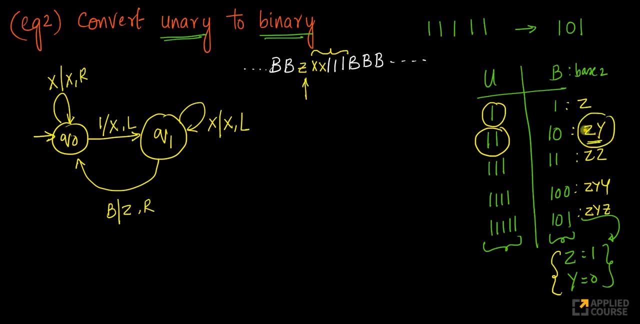 be. My output should be ZY. I have a Z here Right. Look at this. This is where I am moving left. This is where my output is Right. This is where my output is. This is where my input is. This is. 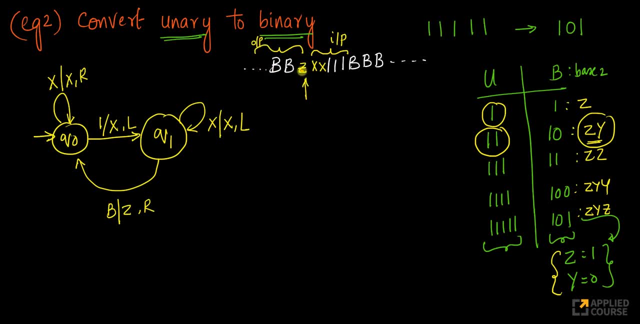 where my output should be. Now I have Z, So I should replace this Z with Y, Right. So replace Z with Y and keep moving left, And keep moving left, Right. So now what will happen here? Because this Z has been replaced. Look at this: This Z has been replaced by Y. 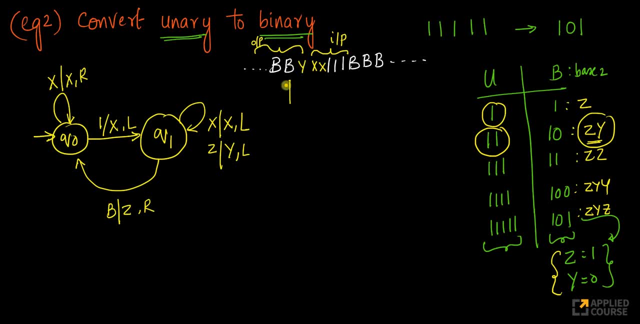 This Z has been replaced by Y And I am moving left because I need to still place my Z here. My output here, because I have read two inputs here, because I have read two 1s and I have marked these two 1s as X, my output should be ZY. My Y is there Now B. Look at this. This is cool. 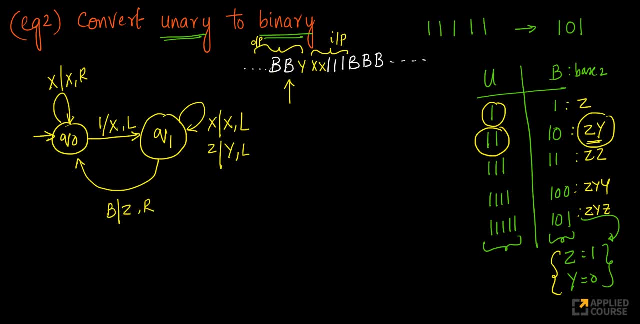 B should be replaced by Z and move right. Cool, So B will be replaced by Z. I already have the transition: B will be replaced by Z and I am going to move right. Right, So now I will arrive here. 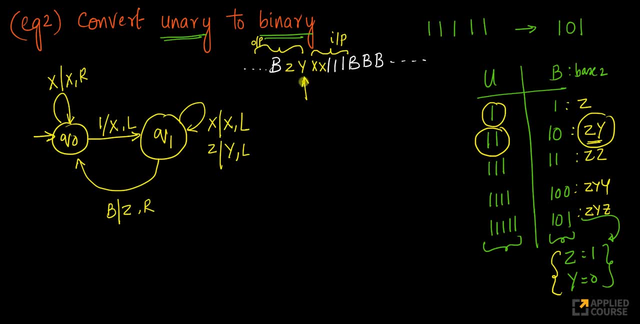 Now I will arrive here. Cool, This is good. What should I do here? I should not touch this. I should not edit this in any way. I should leave it as is Till the time I reach 1,. I should just not edit this, Because I have read. 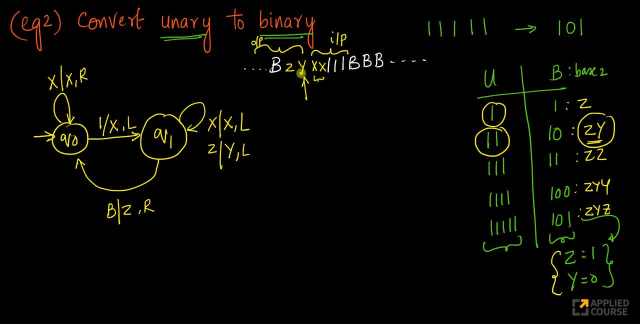 two 1s now and my output also corresponds to the binary equivalent of it, which is 1,, 0 or Z? Y in our context. So here, what will I do? here? Y just leave it as is and keep moving right, Right, So? 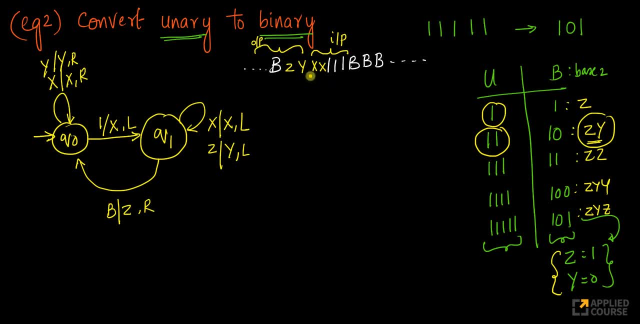 just leave your Y as is: Keep moving right. Now I get an X. Keep moving right, X, keep moving right Till the time I get 1. now Look at this: Now, when I get 1, what should I do Again? are all transitions done? We don't know. Let's run through the whole example. 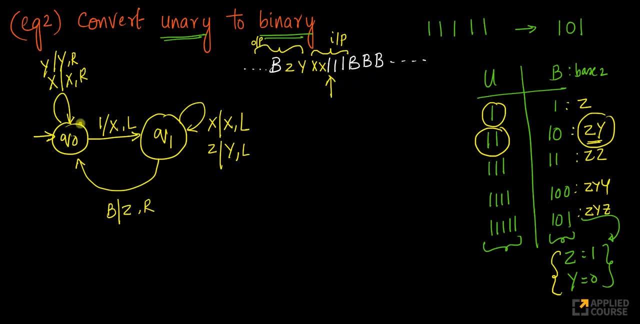 Right. So when I get 1 here, what should I do? 1 will be replaced by X. Cool Right. 1 will be replaced by X. So let me just replace this 1 with X, and I am going to the left. When I go to the left, what happens? I keep replacing my Xs with. 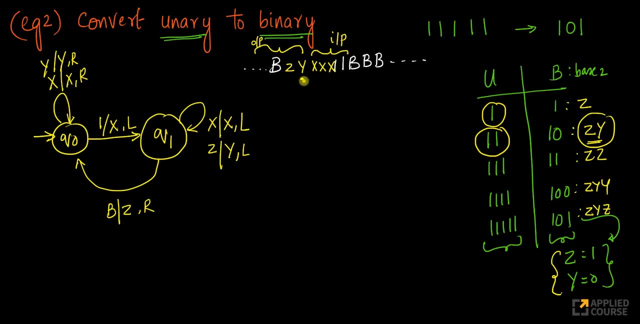 lefts. I keep replacing. Now I reach here. Now, look at this. Now I reach here. Now. what do I want? I want Z, Z. Now, what do I see here? If you notice, what do I see here? I see a Y. I see a Y, This Y, now Look at this. 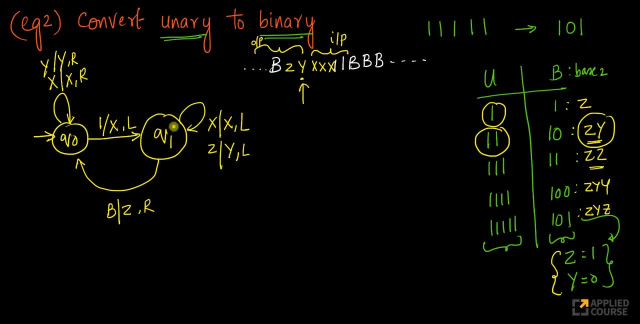 This X replaced with X. I have reached here now, Finally, And my state is still q1.. Now I have Z Y, Because I have read 3, 1s. It should be Z, Z, So this Y should now be replaced with. 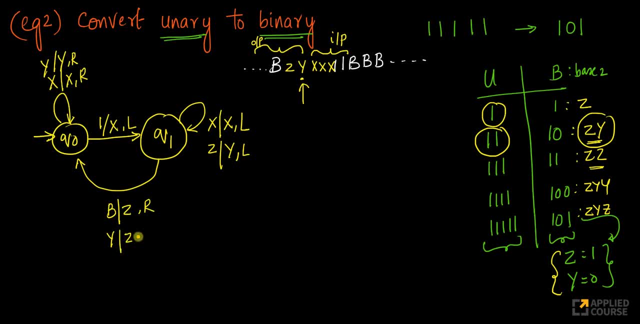 Z. Right, This Y should now be replaced with Z And I can keep moving right. Then I don't have to worry. So if I just move this to Z, look at this. if I move this to Z, I am done. I have already accounted for this. 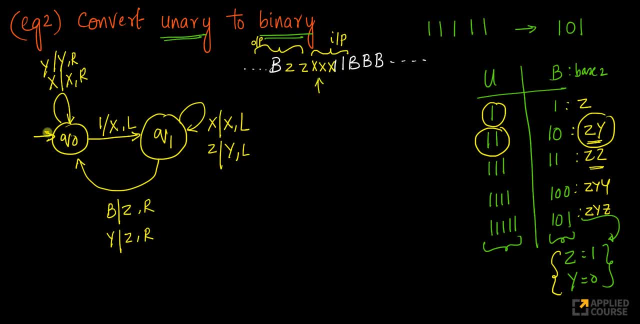 and I keep moving right now. Again, same. all these transitions will play a role. Everything Now let us keep going forward. Now what will happen here? If you notice this X, if I keep getting Xs, keep moving to the right. When I get a 1, replace that 1 with an X. Look, 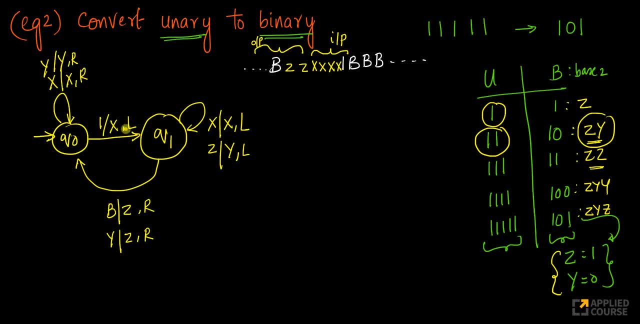 at this: this X, I will replace with this 1, I will replace with an X, and I will go to the left. And now, if I keep encountering Xs, I will keep moving back, If I keep, if I encounter a Z. now look at this. Now I have read 4,, 4 ones. What should my output be? 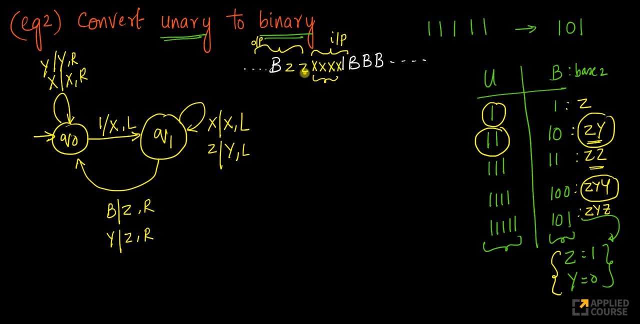 My output should be ZYY, So this Z will now get replaced, because I am in this state right? Look at this. this Xs got replaced with Xs. I am moving left here. Now I am in this state. This Z will get replaced by Y. This Z will get replaced by Y Again. this Z also will. 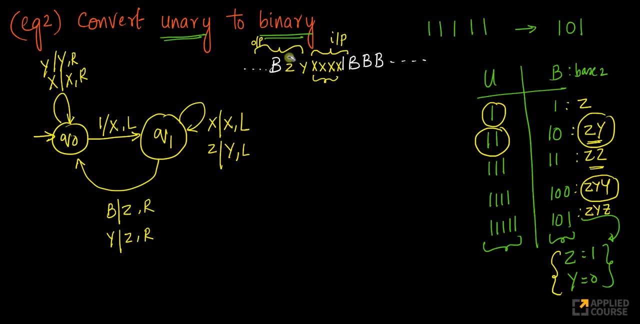 get replaced by Y, This Z also will get replaced by Y. This Z also gets replaced by Y, Then this B should get replaced by Z. So this, this will become Z now. So let me erase that and write it down. So this, so this will become Z now. So now I have read 4 ones and my output represents: 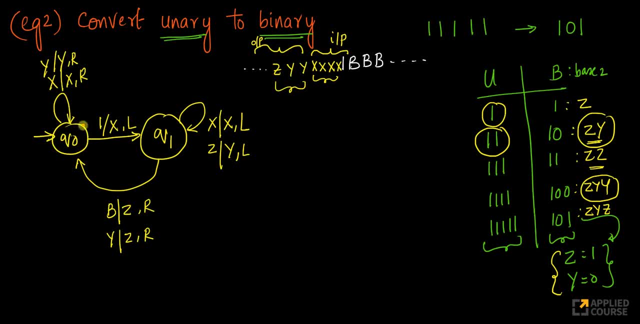 1, 0, 0.. I am still in again in state Q0,, right? So look at the whole flow Now I will again if. if I keep getting Ys, I will stay here, Right. If I keep getting Xs, I will stay here till the time I get 1.. Finally, when 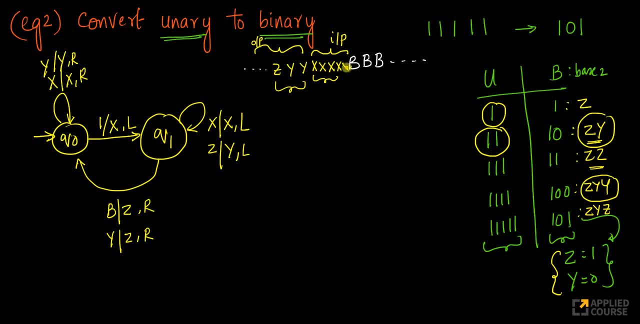 I get a 1 here, what will I do? I will change this 1 to X, I will change the 1 to X and I will keep moving left. Look at this: I keep moving left. Now, what is the corresponding value of this? Corresponding value of it is ZYZ. Now, what am I encountering here? I am 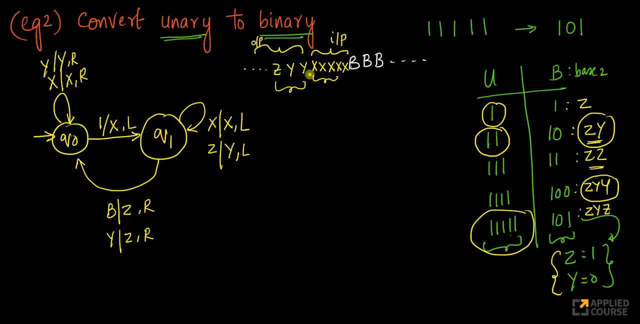 only encountering Y. Now, the moment I am in this state right now, when I encounter a Y, what should I do? I will replace the Y with Z. Look at this: I replace this Y with Z And I keep moving right. Right, That is it. I keep moving right. and now, finally, what will? 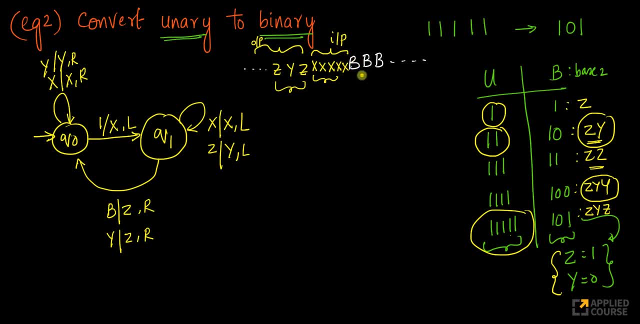 happen, I will encounter a B. Look at this. finally, I am encountering a B, Right, There is nothing else left. So when I encounter a B, what should I do now? So now, everything is processed. I am left with B. now, Right, I keep going forward. Now I am left with a. 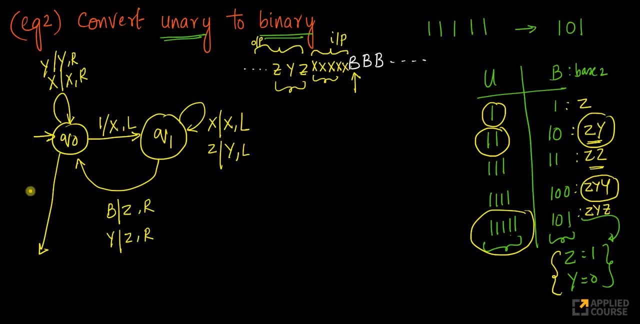 B, No more 1s left, Right. So I will create this one more transition here and say: if I encounter a B, keep it as B itself, Right, Keep it as B itself, Then move right and I will move to a final state here. Right, I move to a final state. 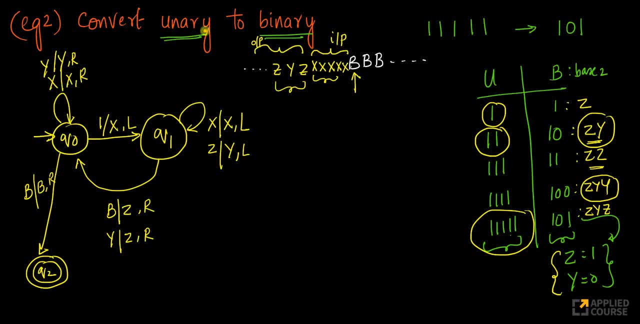 here. That is it. That is all. That is how you convert from unary to binary. Extremely simple. Again, this is very easy to do it with some examples. Again, the strategies that we learned when we started designing finite automata, wherein we take a bunch of 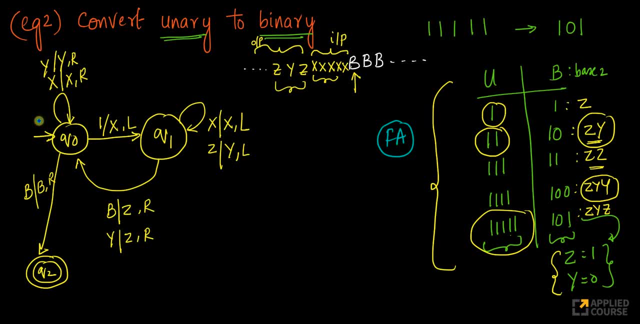 examples, this whole state transition. the only fundamental difference between your Turing machine and finite automata design is same example based approach you will employ here. But just remember how you are changing the symbols from one symbol to other symbol and whether you are moving left or right. So that is why we focus so much on finite automata. 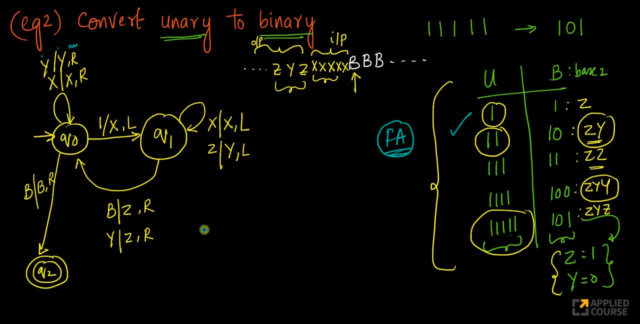 design, Because, if you understand this, designing other forms of automata becomes much more easier, Right? So this is one. again, this is a very, very important task, Right, Converting unary to binary Only. again, this is like an input-output device. This is not about. 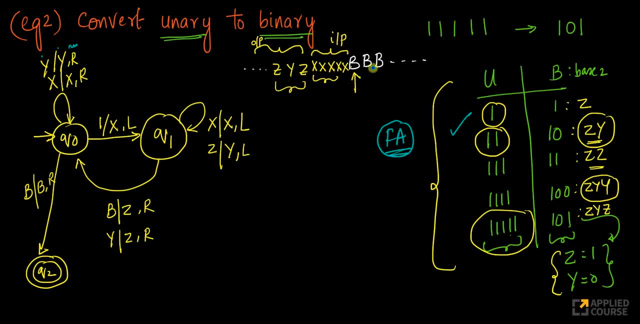 language acceptance Here. what do we have Here? this task is not about language acceptance. This task is about a computer with input-output. Right, This is a computer with input. Given an input, we are generating an output. This was the input that was given to me. I generated. 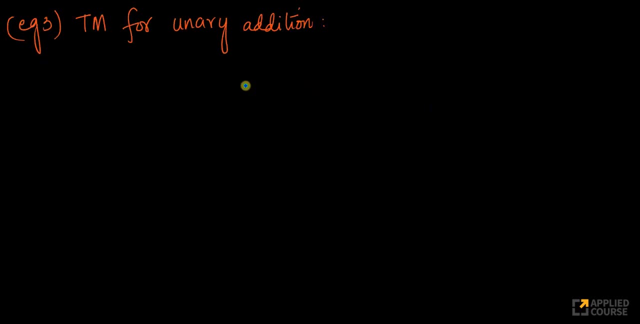 the output Right. So very interesting approach here. Now let us look at one more thing Right, One more problem here Again, I will also point you to many, many other resources. I will show you some examples and explain them in detail, But I will also give you more resources. 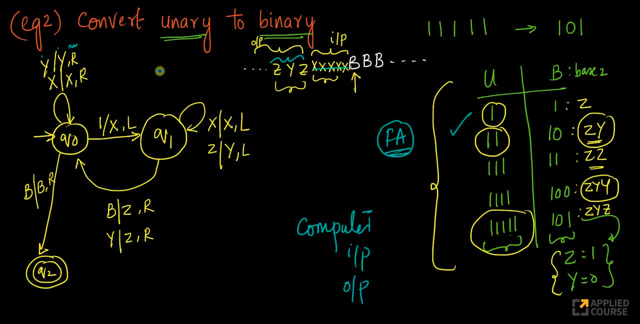 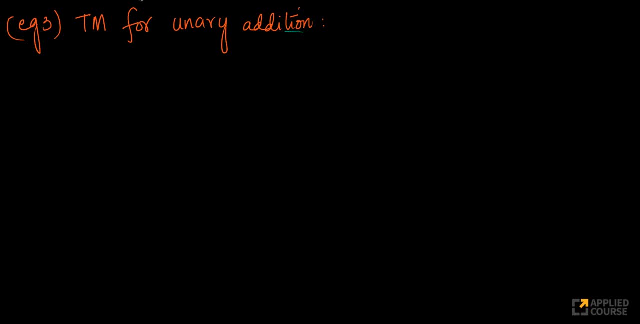 so that if you want to look at more architectural designs of Turing machines for other problems, you can go through them Right. So Turing machine for unary addition. So let us say how the input should be. first Let us discuss about the input. Again, here I have unary. 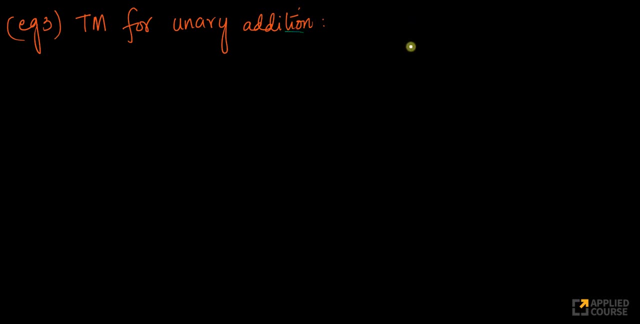 addition, which means I have two unary numbers and I want to add them. How can I input that? Look at this. I can input it like this: I have two zeros followed by a special symbol C, which you can think of it as a separator. So this represents two, And I have blanks. 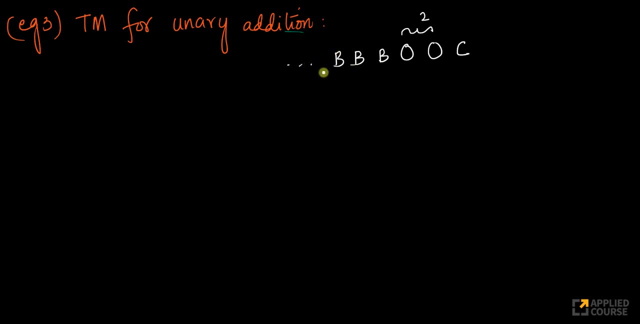 here. Look at this: I have blanks here. All of them are blanks. Right, I have a C Blank. then I have zeros here. So this represents unary. 3. This represents unary 2. Here I am using zeros instead of ones. Right, You can use any symbol in unary. You can use A also. 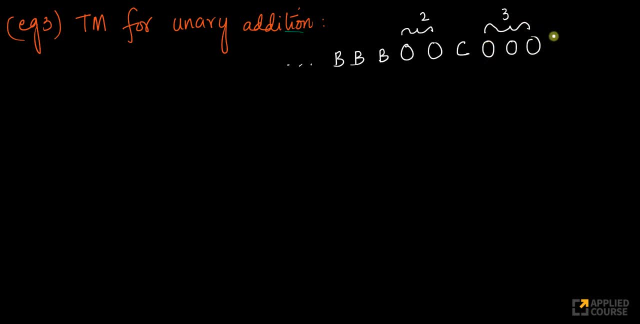 So there are two zeros here and there are three zeros here And I want to add them Now. I have all blanks Right. Look at this. This C is a special symbol that is used as a delimiter between your unary 2 and unary 3.. You can use C, or some people also use plus. 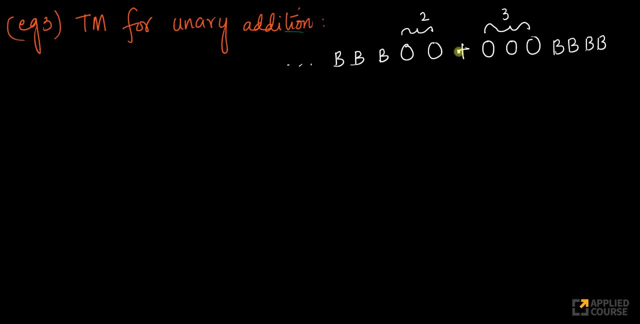 symbol here, Because plus is also a symbol. Plus is also a symbol. I just need to have my plus as part of my tape alphabet. If I have my plus symbol as part of tape alphabet, I am done Right. So here you can place any symbol here, like a plus symbol or anything. You can place any. 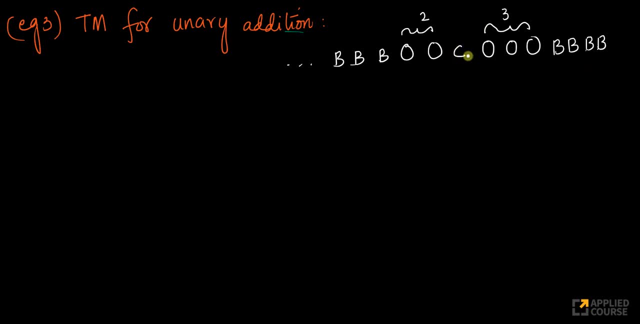 symbol. We will go with C, Right C, basically implying that C is a separator between my unary 2 and unary 3.. What is the output that I want? Look at this. What is the output that I want? I want my. 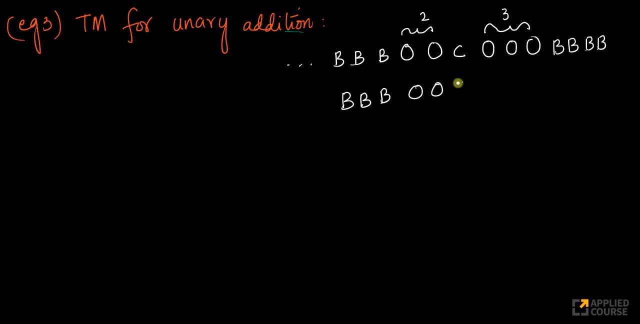 output to be BBB Five zeros. Right, Five zeros, Because this is addition. Right, Two plus three is five. This is what I want. Right, And then I want BBBB, so on, so forth. Right, This is what I. 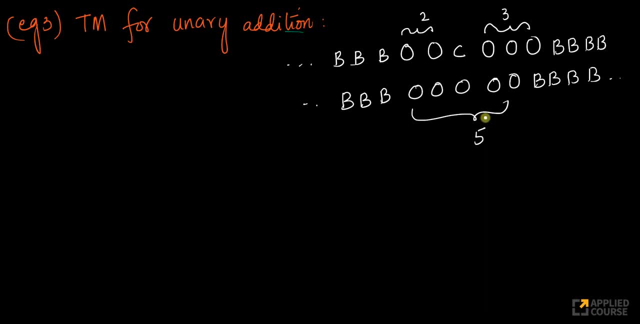 want to achieve. How do I design the finite? how do I design the Turing machine for this? Not finite automata, Sorry. So let us keep going with this. So let us keep going with it, step by step. Now, what we will do here, instead of this type of arrangement, let me tell you the idea. first, I will tell 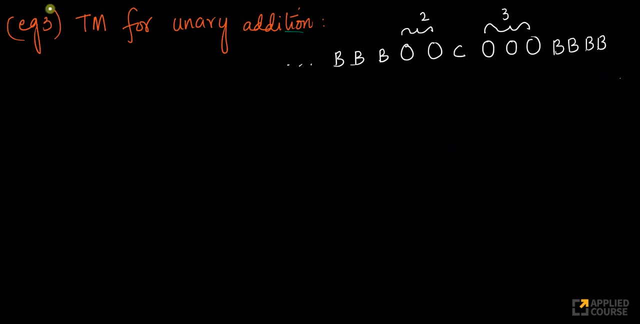 you the idea, Then we will design the Turing machine itself. So what I will do? I want five zeros as my output, But the way I will go about it, there are multiple ways of solving this problem. What I am showing you here is one approach. Just a while later, I will also show you another. 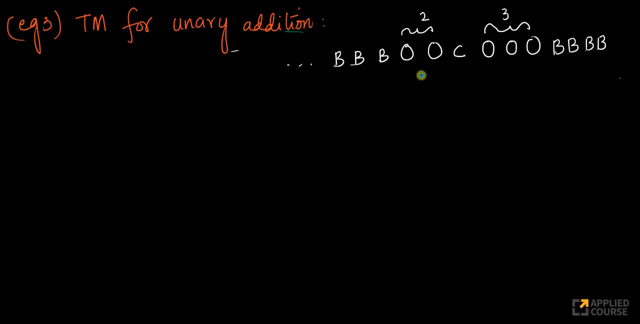 approach of thinking about it, Just to show you that there are multiple ways of thinking about it. So what I will do, my input will. I will start reading my input from here, Right, I will start reading. So whenever I encounter a zero, what I will do here. look at this, what I 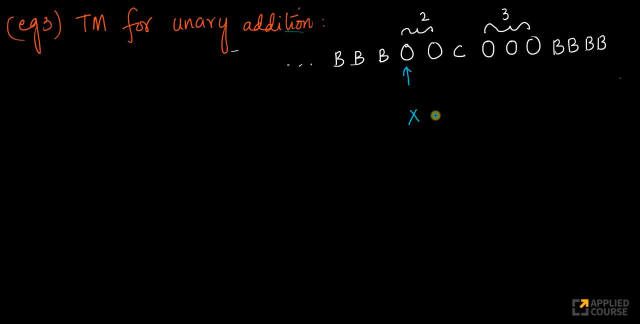 will do here is: I will just make it an X Right. When I make an X out of it, I will make an X out of it. Look at this: What is my input tape right now? My input tape is this: I am just aligning everything Right. So when I read a zero, what I will try to? 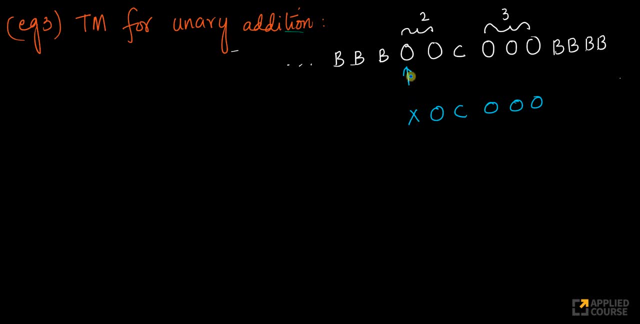 do here. what I will try to do here is I will keep my zero as is. I will- sorry, I will change my zero to X and I will place a zero at the end of three. So I am converting the zero to X and I am placing a zero after the zero. So this stays here. this stays here. 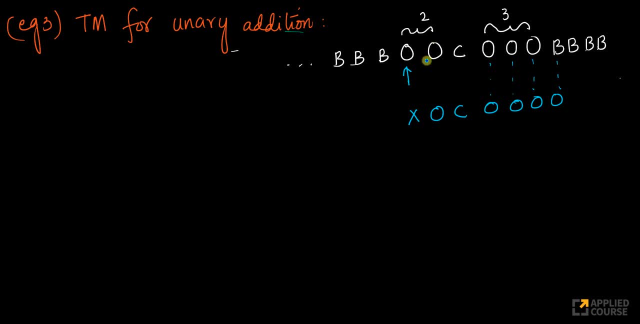 this stays here. Instead of this B, I will place a zero. Similarly, I will take this, I will move. I will convert this into an X. Look at this. I am converting this into an X, Right, And then I will add one more zero here instead of a blank. Now, if no more zeros, 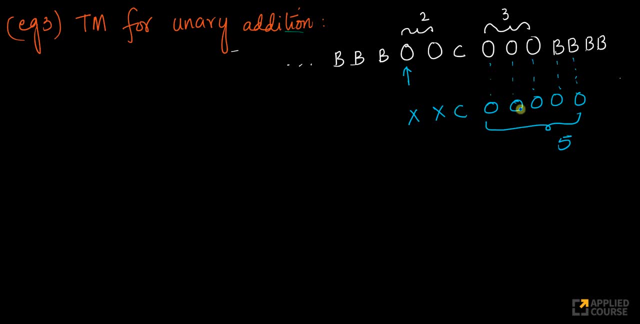 are left. what I am left with here is equal to whatever I am left with here, which is after: this C Right Is the unary addition equivalent Right. It is a unary addition equivalent Right. So this is one strategy of doing it. So let me write the Turing machine. 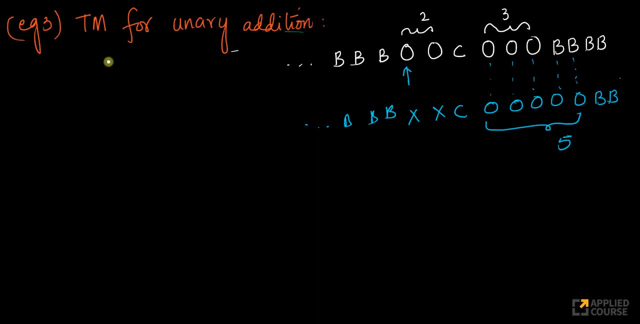 this. We'll start with this example. This example should be good enough for us to construct the whole Turing machine. So I'm in state q0. Let's go with it. So I encounter a 0. The first 0 that I encounter, I'll replace it with x. So when I encounter 0, I'll replace it with x, and it'll. 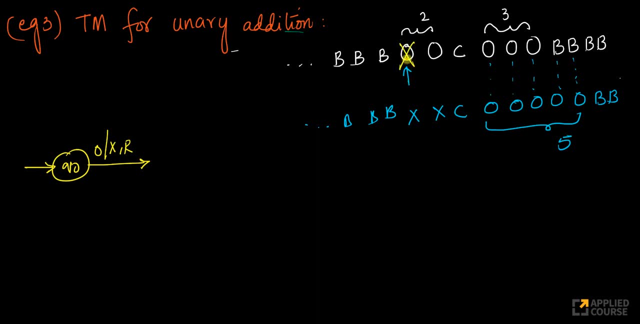 keep moving right. So this 0 has been now replaced with x. Cool, Now I move here. Now, if I encounter more 0s, I won't do anything. Look at this: If I encounter more 0s, I let it be as is, because I. 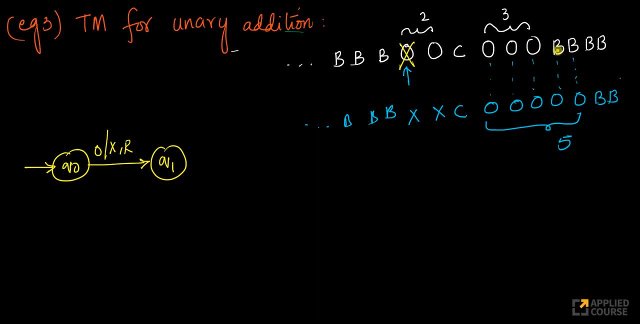 only want to make one 0 as x and place a 0 here. Then I'll come back, make this 0 as x, place a 0 there, and so on so forth. I want to do it step by step. So if I encounter more 0s here, I will not. 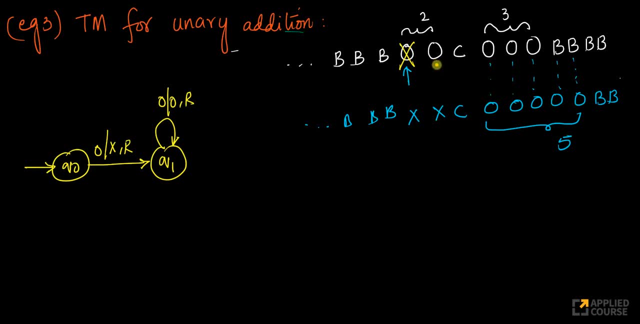 touch it. I'll just keep them as is till the time I encounter a c. Look at this. So now, what happens here? So this is red. Look at this. This is done. This is done Now. I've moved to c here. Now, when 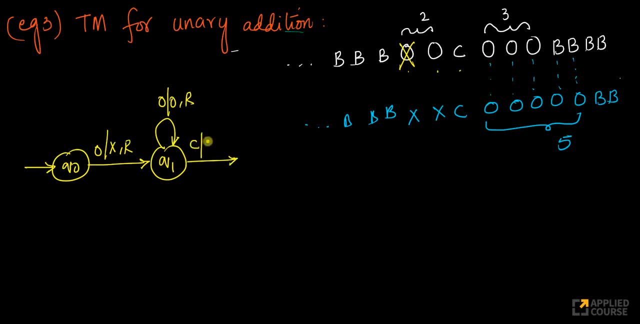 I encounter a c, what should I do? Keep the c as is, Don't touch The c, but move to the right. And I'm going to a different state here to know that, yes, I've already read, I've already moved over from c. Now here, if I encounter 0s, I don't want to do. 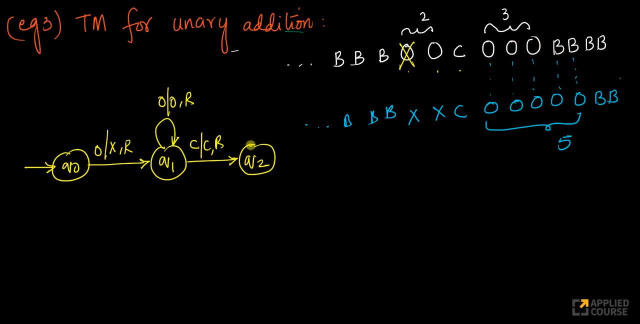 anything. Only when I encounter a, b, I want to replace it with 0. So here, if I encounter 0s, I want to just keep them as is. So I keep moving to the right Now, when I encounter a, b, look at: 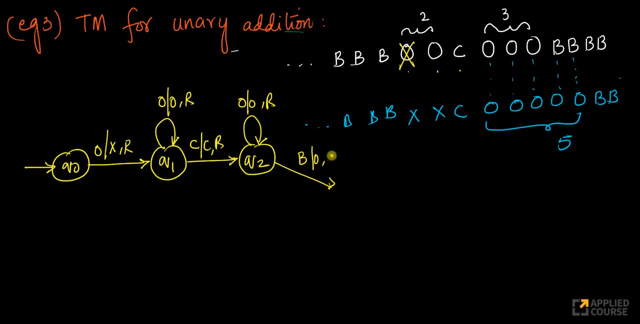 this Now: when I encounter a b, I want to replace it with a 0.. When I encounter a b, I want to do this with a 0 and I want to start moving left now. Right, I want to start moving left now, Now. 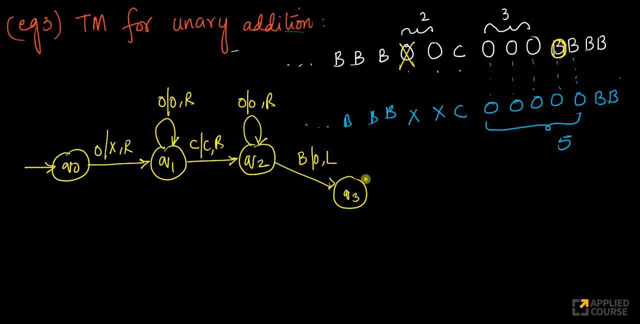 when I'm moving left. now, if I encounter 0s, look at this. If I encounter 0s, I'll just keep them as is and keep moving left, Right. If I encounter a c, look at this. If I encounter a c, what will? 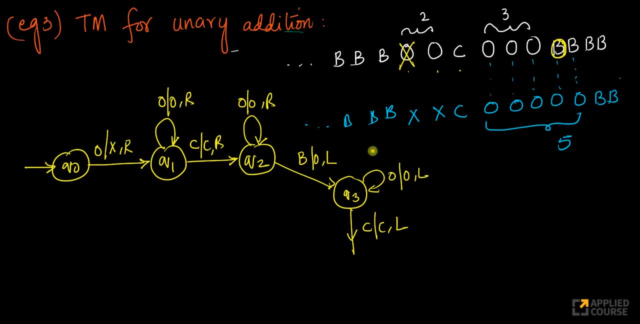 I do. I'll just keep moving left. Don't touch the c, Keep moving left. So this state basically means that I've seen 0s, I've seen the c also. Now I've come to the other side. I've come to the other. 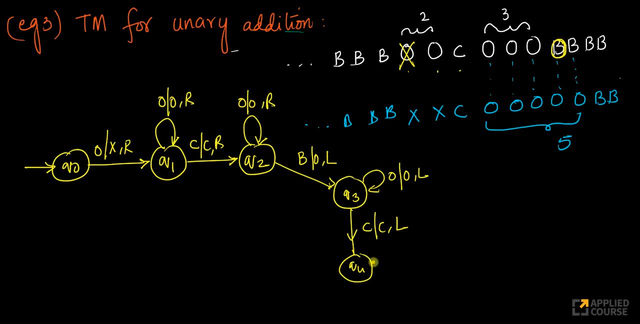 side of c. That's what this state says. Now, from this state: if I keep encountering 0s, look at this. If I keep- suppose there could be more 0s also here- right, There could be more 0s- I'll leave the 0s as is. I'll leave the 0s. I'll keep moving left. 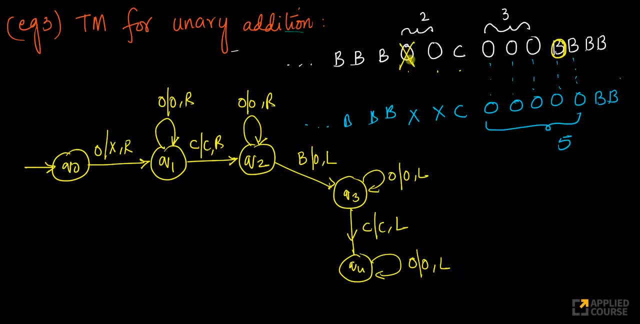 But when I encounter an x, this means that, okay, no more 0s to the left of it, Right. So when I encounter an x, what should I do? This whole process that I've done should repeat. So what I'll do here is this: So when I encounter an x, now I'll keep the x as is, but I'll move right. 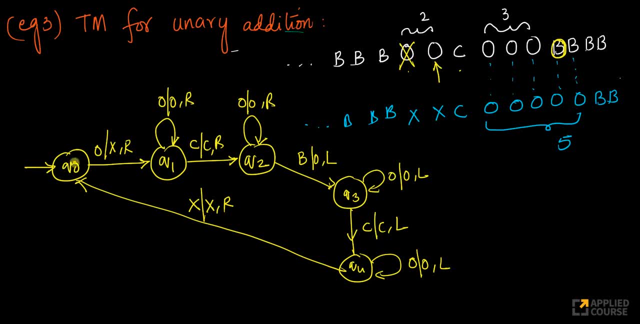 Now I move here. Now this whole, what is this whole cycle doing? This whole cycle is taking a 0 here, replacing it with x, move forward, replace this 0, replace this b with a 0 and keep and come back here, And that's what this whole cycle is doing. So if I repeat the whole cycle, what'll? 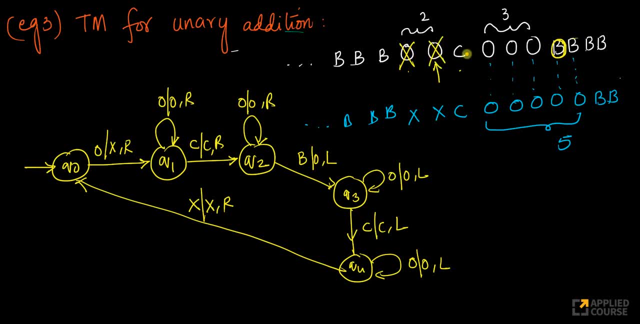 happen. This will become x. It'll go forward, c, nothing, Keep going forward till the time it encounters b. When it encounters b, it'll replace this b with 0 and it'll start its trajectory back. Once it moves back, what happens Finally? I'll reach here Right, This whole loop, this: 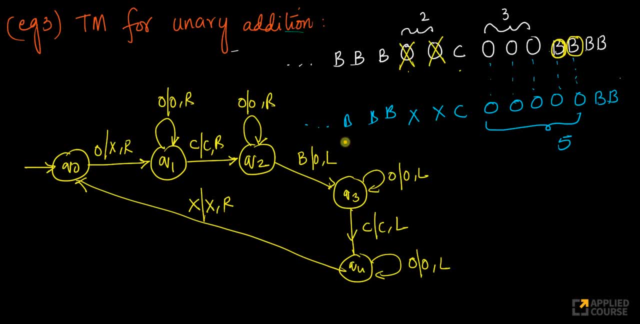 whole loop, finally. So this, this whole part- x, x. when I encounter x, I'll keep the x as is and I'll move here. Once all of my input is over, what happens? Look at this, When all of my input is. 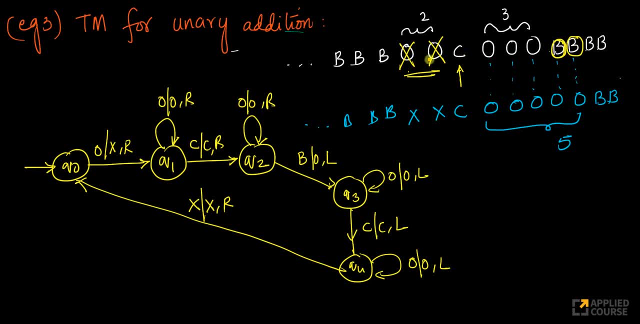 over right. When all of my input is over, I'll encounter c. No more 0s left here, Right. So when I encounter c, what should I do? I should change my c to b and move right and go to a final state. 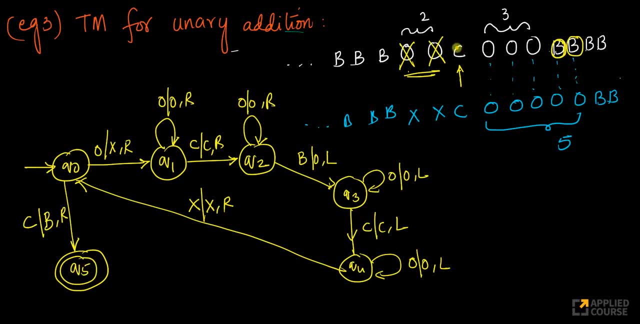 Right. So this becomes my final state. So what do I do now? This c, I'll convert it into b. So this c, I'll convert it into b. Right Now, what do I have? Look at this, What do I have? I have: 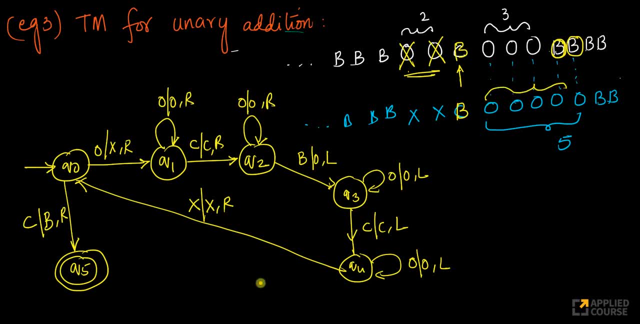 my five 0s that I want here Again, this is one of the Turing machines for unary. addition, We can also design other Turing machines also. And look at how we design this Turing machine Again. we first design a logic. This is: this is: this is the. this is one of the possible logics for unary. 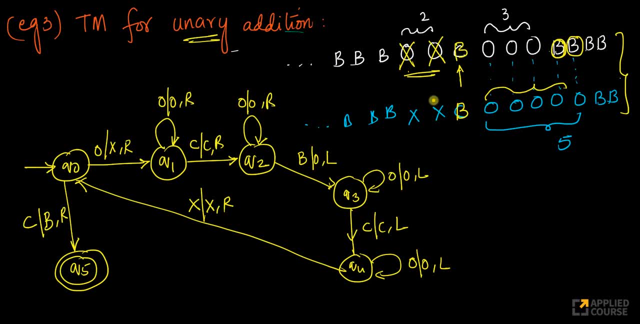 addition. I'll show you one more logic so that you understand. So this is one of the possible logics for unary addition. I'll show you one more logic so that you understand that there could be multiple logics or multiple ideas on how to construct Turing machine. Once we get the logic. 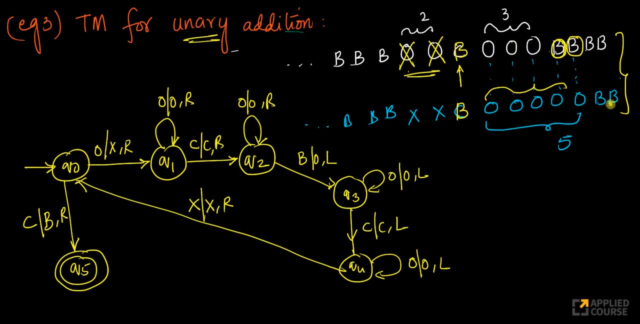 once we think of the basic logic on where the input should be, where the output should be. how should we work? Again, remember that this is an input and output machine. This is an input and output Turing machine, because we're giving it two inputs and we're getting an output, And then 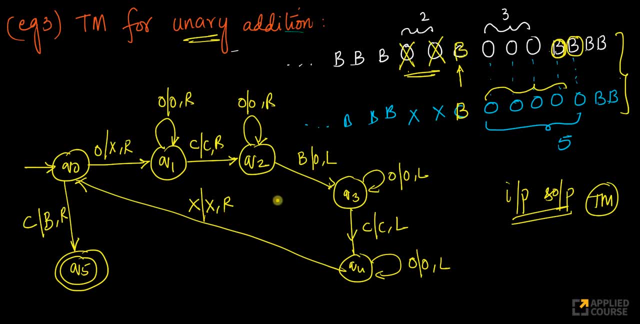 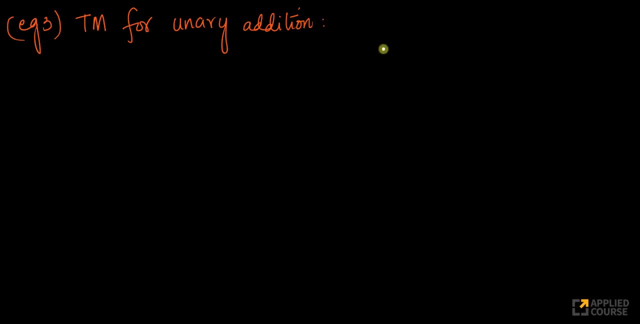 designing all the transitions and all is straightforward if you are just using examples to construct it, Right? So let me show you one more way of doing it. So Turing machine for unary addition with a completely different logic. Okay, So here here, let's assume I have 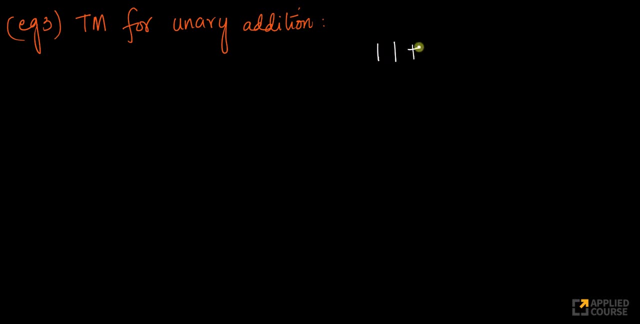 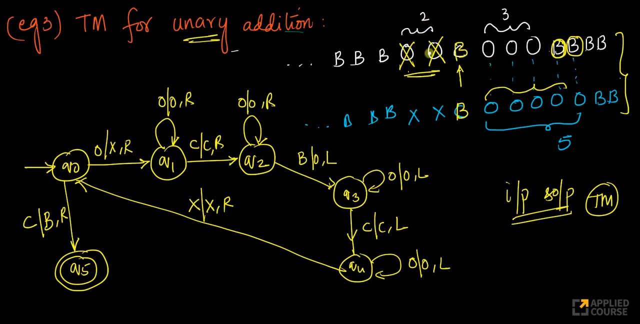 one one. Look at this. Imagine I have my tape consists of these symbols Once Again for unary. all these are blanks. All these are blanks Right Here, if you notice, my unary two is represented using ones. Again, I can represent using zeros or ones, Doesn't matter. Okay, My 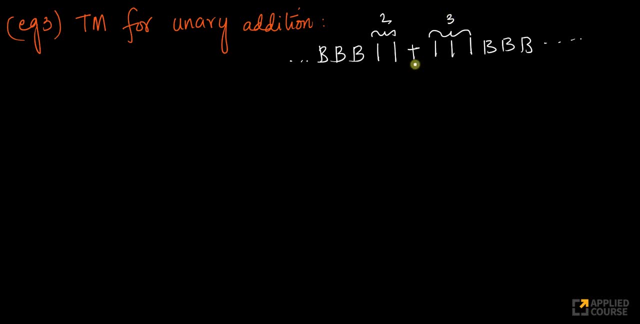 alphabet changes. That's it, This is three, and I have a special symbol called plus here. Now let's see, Let's see one more strategy of doing it, One more idea of solving this problem is this: What I'll do here is: I'll keep the B's, as is Okay. I'll keep the same, I'll keep the tape. 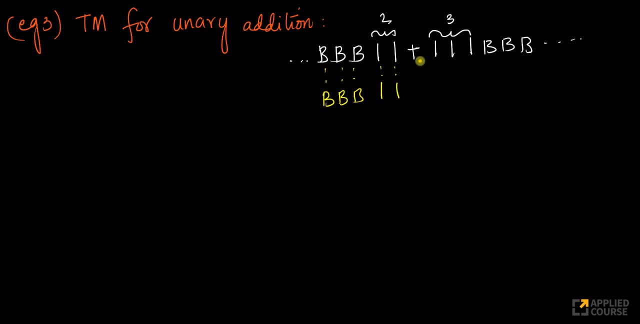 symbols, as is. I'll keep this one also, as is. I'll keep this one also as is. I'll change this plus to one. Look at this: I'm changing this plus to one and I'll remove this one. This one stays. 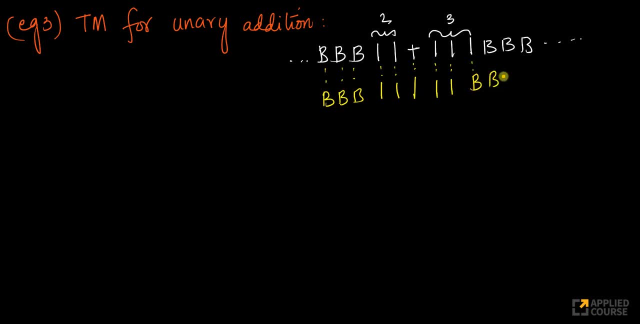 the same. This one, this one, I'll make it as blank and the blanks stay the same. So what am I doing here? I'm just changing the plus to one. Okay, This is an other strategy. Right Again, here you see this. You have two, you have three. 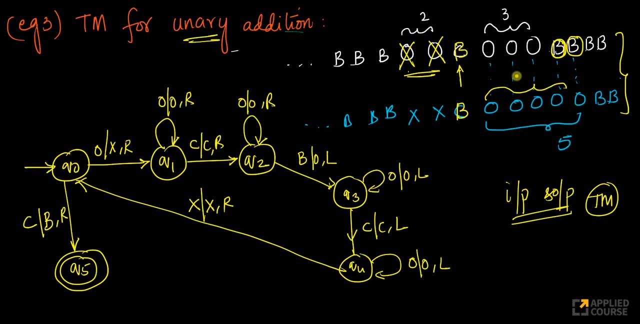 and you have five here. This is another strategy that I can employ. What we saw here is one strategy where we are taking each of these symbols, converting them into X, going to the very right and placing the symbol there Right, Placing the zeros there. This is one strategy. 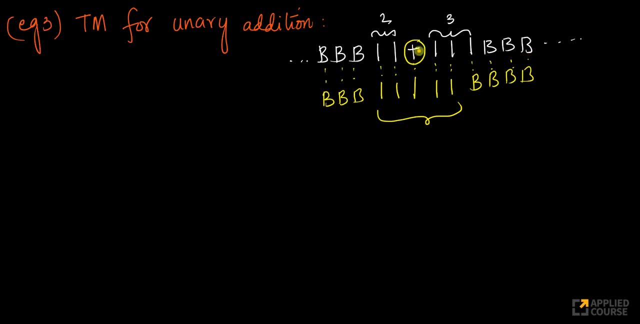 The other strategy, much simpler strategy here, is: change this: whenever you encounter a plus symbol, change it to one. go to the very end. change the last one to B. That's it Now. how do we write the? how do we construct the Turing machine for this? Let's go Q zero. This is where I start. Look at: 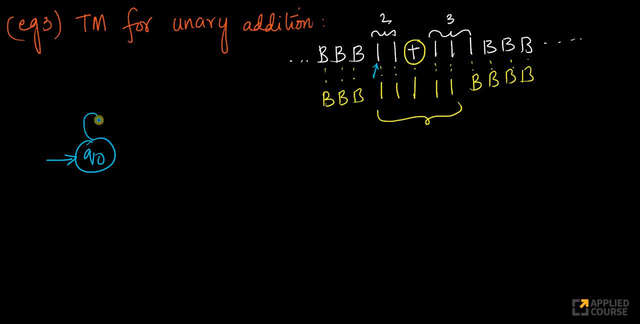 this. I always start here. If I encounter once, just keep moving right, Don't touch it. Okay, Keep the ones as is. Keep moving right Only when I encounter plus, Look at this- Only when I encounter plus, Change the plus to one and keep moving right. So this one has been changed to. 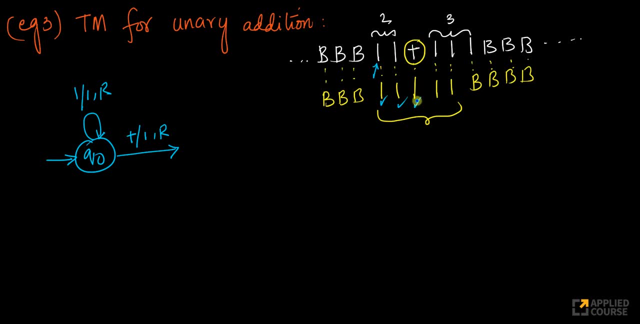 this plus has been changed to one. This is as is. this is as is. this has been changed. Cool, Now I keep moving right If I keep getting ones now. look at this If I keep getting ones now. So let's call this status. 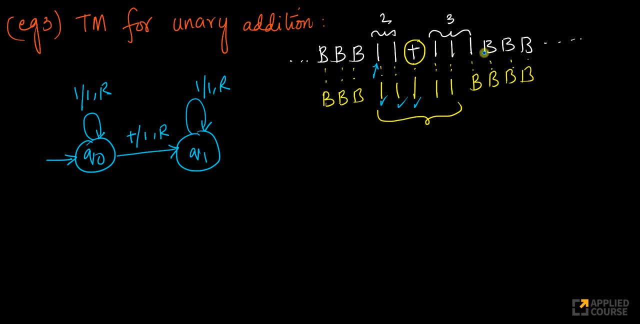 Q one: If I keep getting my ones, I'll keep moving right Till the time I keep getting ones. Finally, I'll get a B. Look at this: When I get a B, I have to go one step back and convert this. 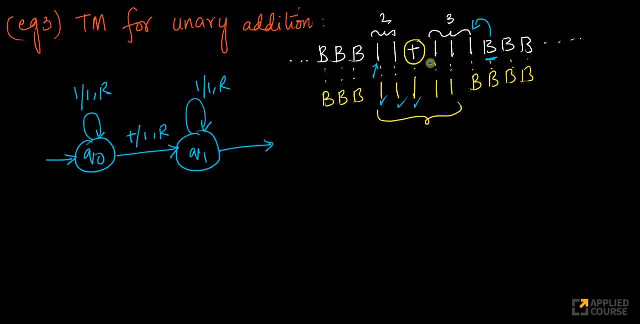 That's what I have to do, right? So if I get a B, look at this Now I'll keep moving. right, I'll encounter a B somewhere. If I get a B, keep the B as is, but move left. which means now I have. 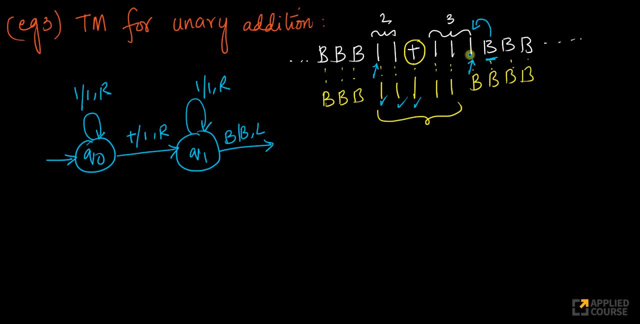 moved here. Look at this: Now I have moved here. This one should now be changed Right. So what will I do here Now? I'll change this one to a blank right. I've changed this one to a blank right Now. what will I do here Now? I've changed this one to a blank. I'll go back. 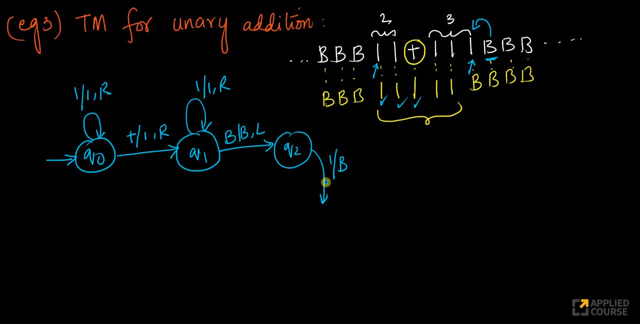 to check whether this is also one or not right. So I'll go left here. Once I go left here, then again I want to check. Look at this: This has been changed to blank. right Now I go back here. This is one right. So this has been changed to blank. So where am I? I'm here. 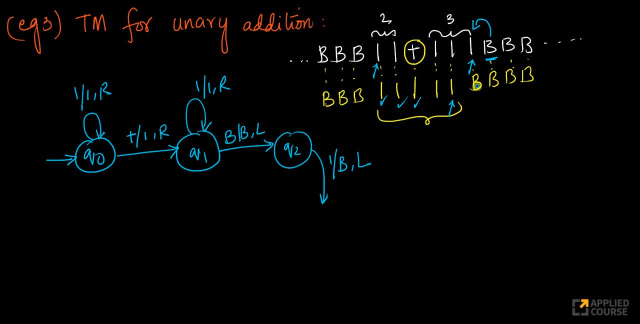 Now I want to see if this is the end or not. Just double checking it here, right So whether this is one or not. So what will I do here? I'll say: if my current input is one, keep it as is. If my 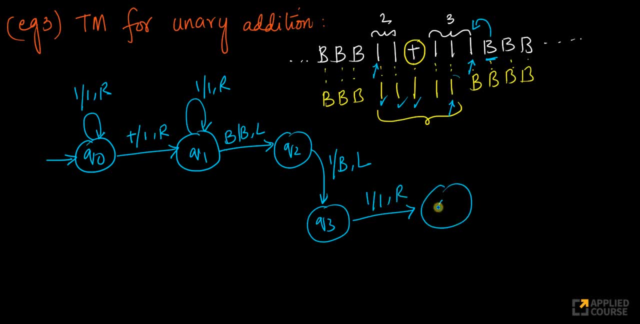 current input is one: just keep it as is. Keep moving right. Now here. what will I say here? I'll say: if my current input is blank, keep the blank as is, and keep the blank as is, Move right and just accept it. That's it. Look at all the steps that I'm doing here. 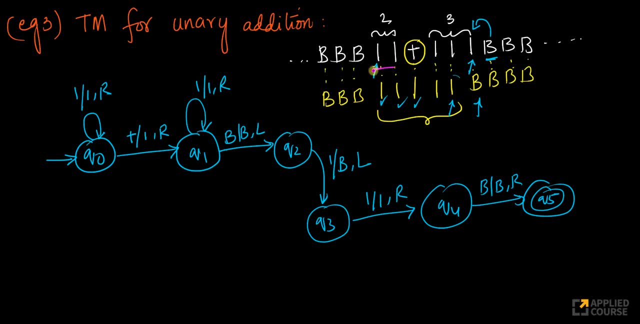 Okay, Step by step again Okay. So if I encounter ones, I'm not touching them, I'm just keeping them as is. That's what this is doing. If I encounter one, I'm changing it to a one If I encounter. 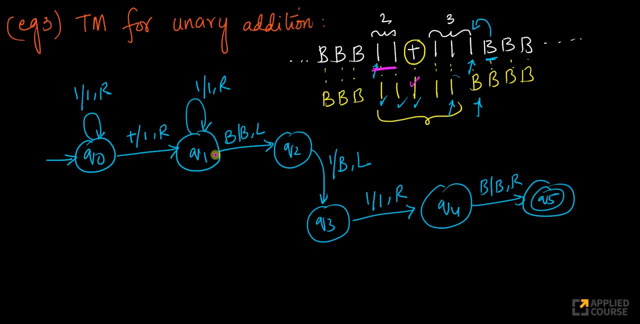 plus, I'm changing it to a one. If I encounter ones, I'm not touching it till the time I encounter a blank. When I encounter a blank, I keep the blank as is. I go to a previous state. Look at this. I go to the previous state because I'm moving left here, right, I go to the previous. 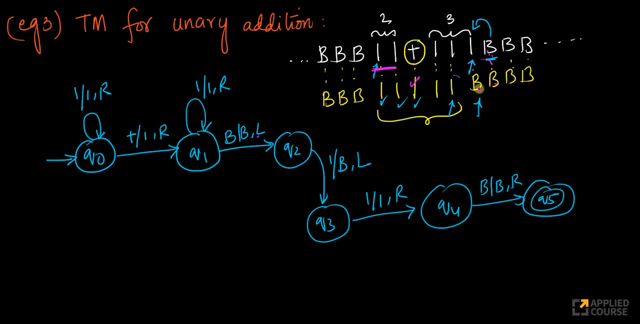 symbol, This previous symbol. if it is one, change it to blank and again move left. Just ensure that this is the last one right Now. if this is one, I go to right and if the next one is B, that means this is the last one. Just ensure that and we reach the final state. 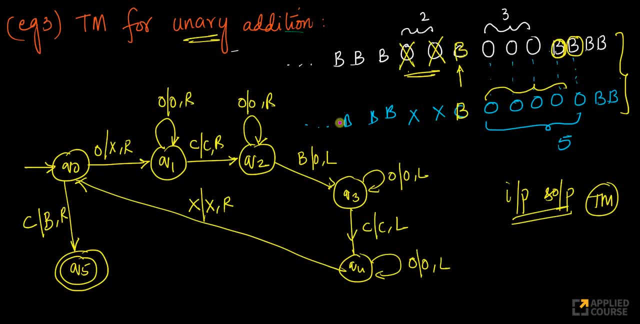 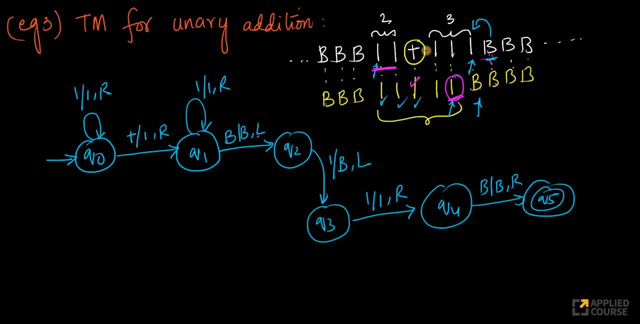 Okay, This is an other. this Turing machine is different from this Turing machine, right? Look at this. Here you have a cycle Here you don't have a cycle here, right? So even if you change the symbols instead of plus, if you write C instead of zeros, 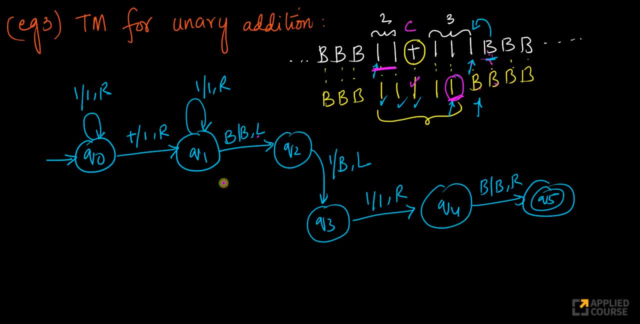 if you, instead of ones, if you write zeros, the whole architecture of the Turing machine itself is different. By architecture, I mean the whole Turing machine Itself is different. By architecture, I don't mean that input. We still continue to have the 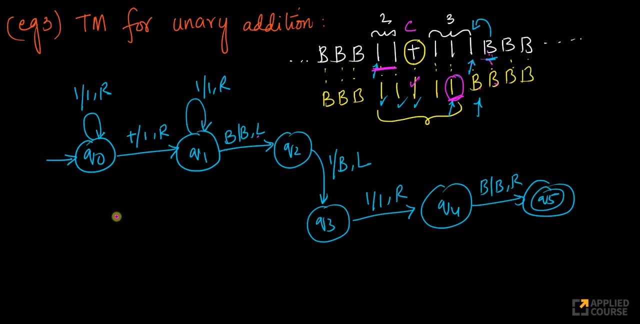 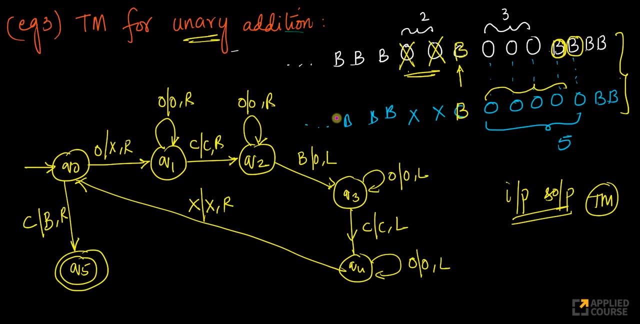 input tapes. We still continue to have the finite control. All of it stays the same. But if you look at the transitions and the states that you have here and the transitions that you have, this is different from this, which means, for the same problem, where you want to perform.